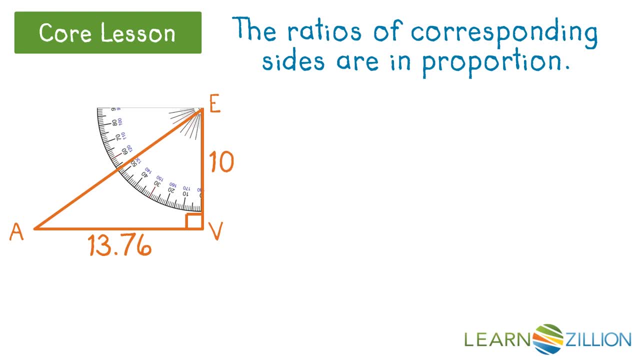 The leg opposite is 13.76, and the leg adjacent is 10.. When we take the leg opposite, 13.76, divided by 10, we get 1.376.. Let's see if this is true for other right triangles. 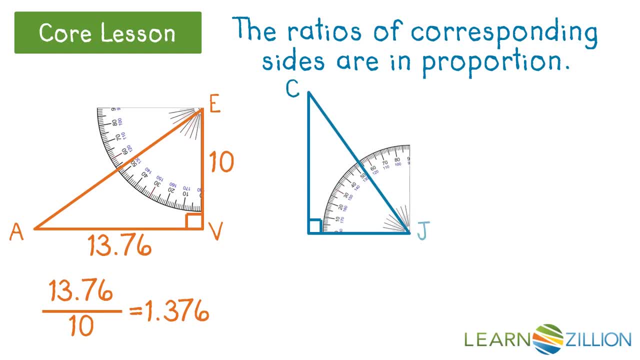 with 54 degree angles. In triangle CJB we have angle J as our 54 degree angle. The leg opposite, angle J is 11.1, and the leg adjacent is 8.2.. When we take 11.1 divided by 8.06, we again get approximately 1.376.. 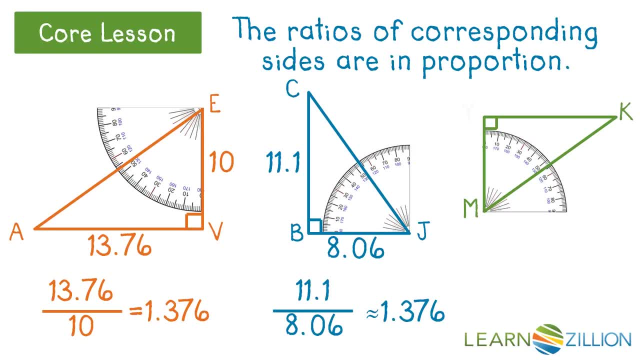 Finally, let's look at a third triangle. triangle KMY M is our 54 degree angle. The leg opposite is 10.32, and the leg adjacent is 7.5.. When we take 10.32 divided by 7.5,, we get 1.376. 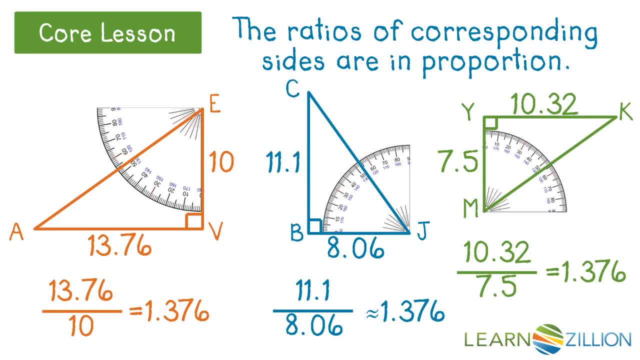 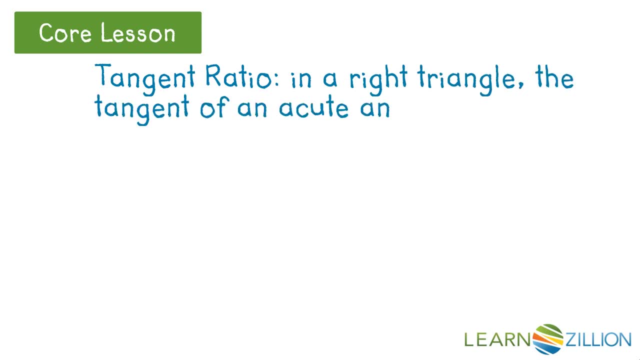 We call this our tangent ratio. The tangent ratio says: in a right triangle the tangent of an acute angle is equal to the length of the leg opposite the angle divided by the length of the leg adjacent to the angle. So the tangent of angle A would be: 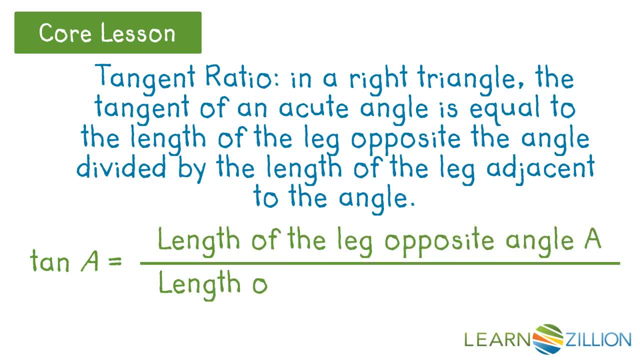 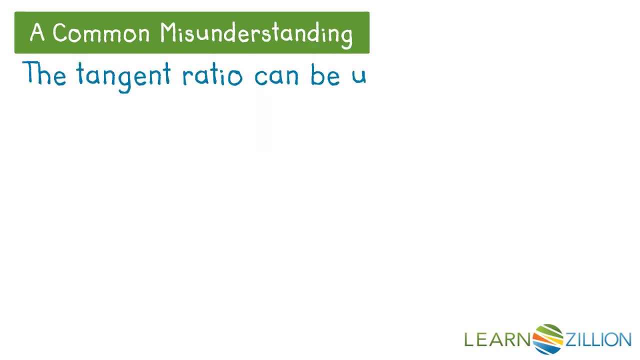 equal to the length of the leg opposite angle A divided by the length of the leg adjacent angle A. A common mistake we make is that we can use the tangent ratio in all triangles. So here we have triangle ABC and you may want to use the tangent ratio in this triangle. 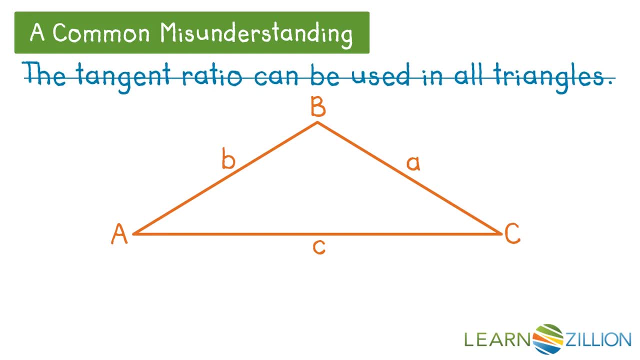 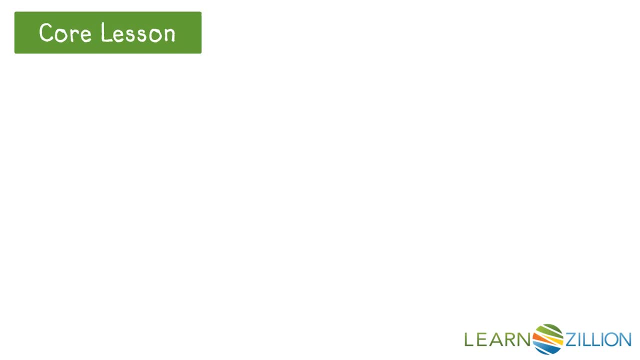 But the fact of the matter is it cannot be used in all triangles. The tangent ratio can only be used in right triangles. A shorter way to remember the ratio is this: Tangent of angle E is equal to the leg opposite angle E divided by the length of the leg adjacent angle E. 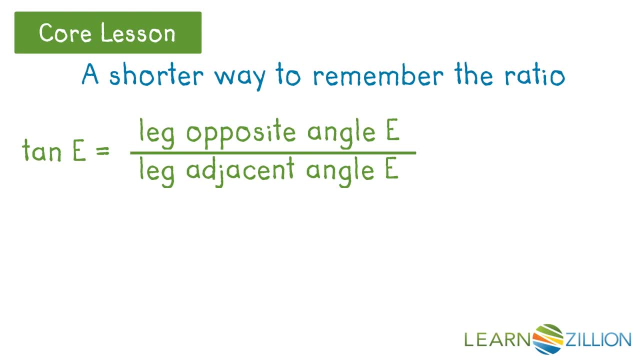 Now you'll also notice that instead of writing tangent when we use it in an equation, we just write TAN. So, looking at triangle AEV, we have our two sides, the leg adjacent and the leg opposite, So we would say the tangent of 54 degrees.